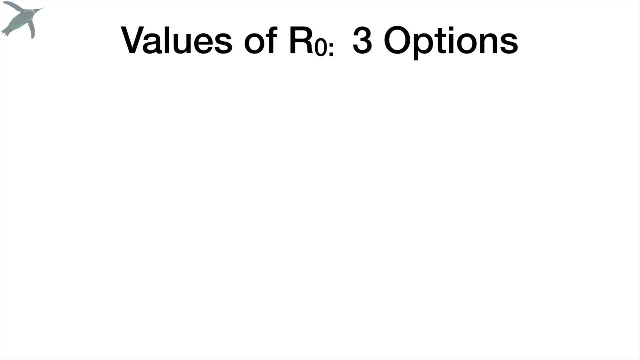 Okay, so those are really important assumptions here. There are three options for the values of R-naught. It can be less than one, which means the number of new cases will decrease over time. That is fantastic. It can be equal to one, which means the case number is stable over time, or it can. 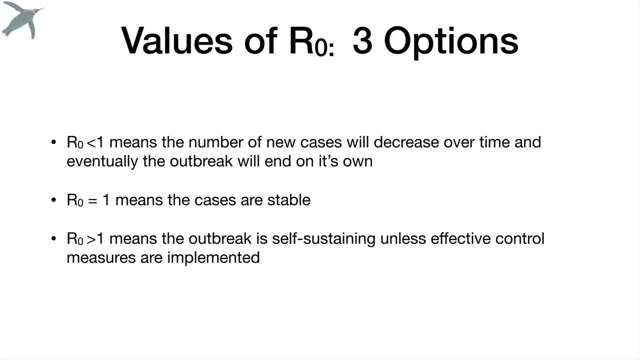 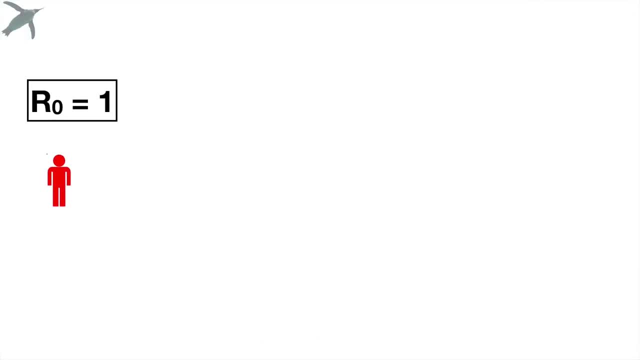 be greater than one, which means that the outbreak is self-sustaining unless control measures are implemented. We're going to look at all three cases in a variety of ways. Here's what it looks like when R-naught equals one. What does that mean? It means that one person infects another person. 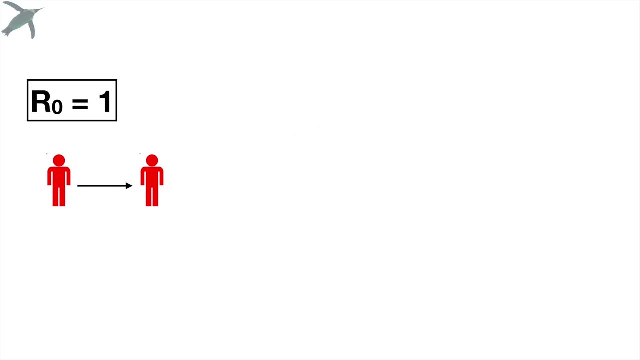 Now, these individuals will either recover, hopefully, or die in a worst case scenario. but each person infects only one other person, So hopefully, what you're seeing here is that the number of cases remains stable over time. If R-naught is less than one, so let's say it's 0.25.. Okay now, obviously humans aren't infecting a. 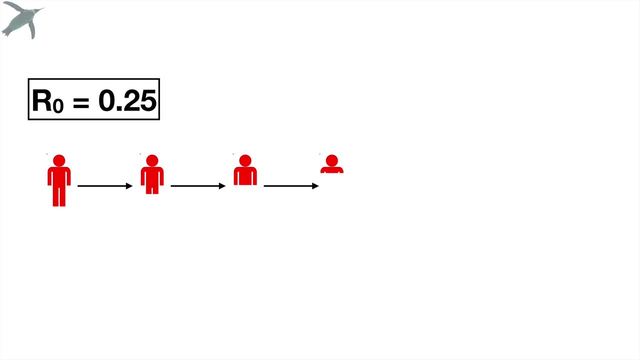 quarter of another human right. This is an average over a population, but hopefully you get where I'm going with this. Over time the number of cases will decrease and will eventually basically die out. That's a good thing. When R-naught is greater than one, let's say R-naught equals two. So when 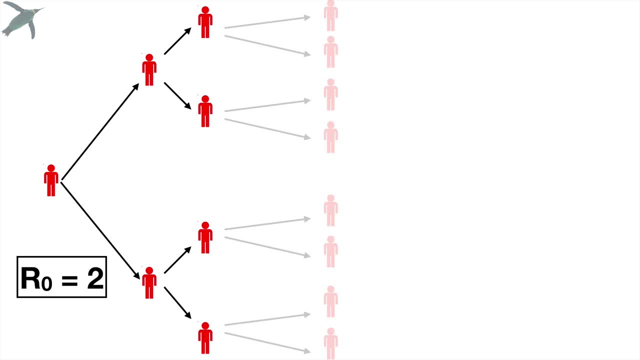 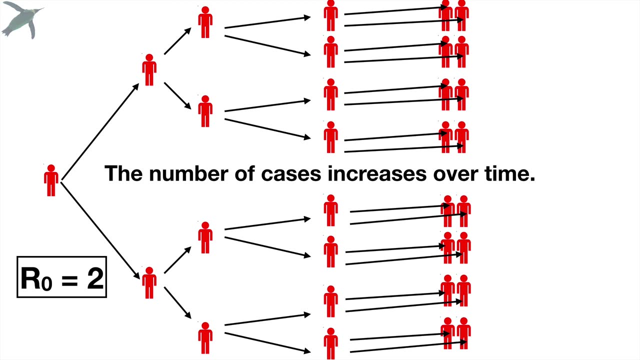 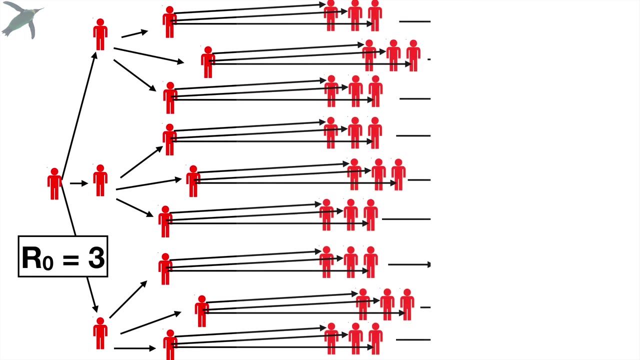 each person infects two people, and those two people infect two people, and so on and so on. you can see how the number of cases will increase over time, And it only gets worse the bigger that R-naught value gets. So here's: R-naught equals three, and things started to get a. 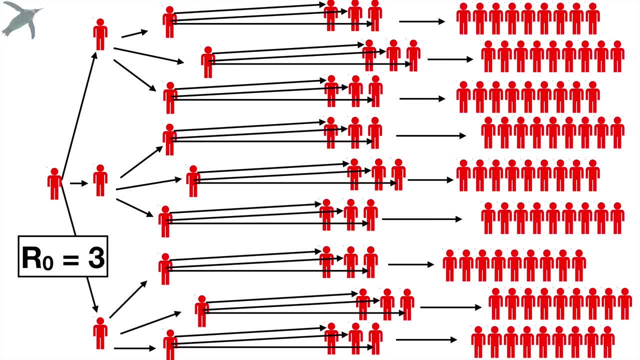 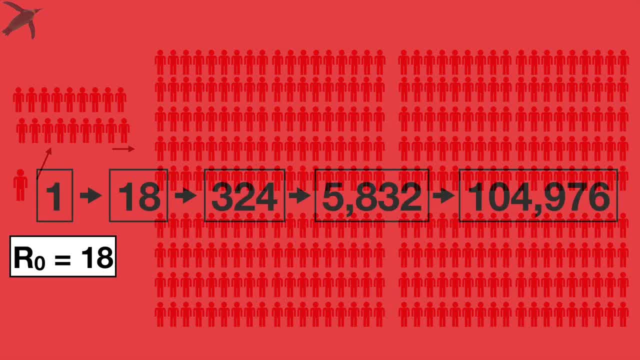 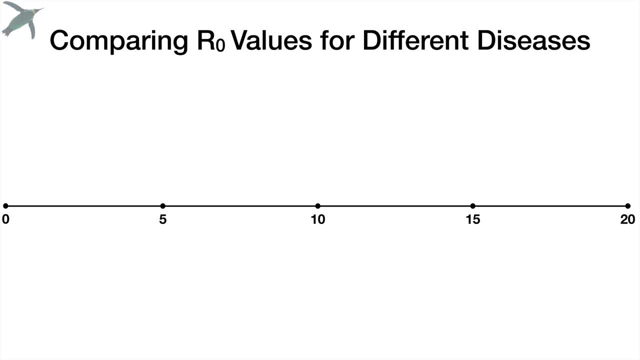 little messy here. Same number of cycles. now I've got 81 people infected. If you look at something like an R-naught of 18- I couldn't do all the generations here. obviously These numbers get very big, very fast. Next, and look at some different R-naught values for different diseases. And, by the way, I got these. 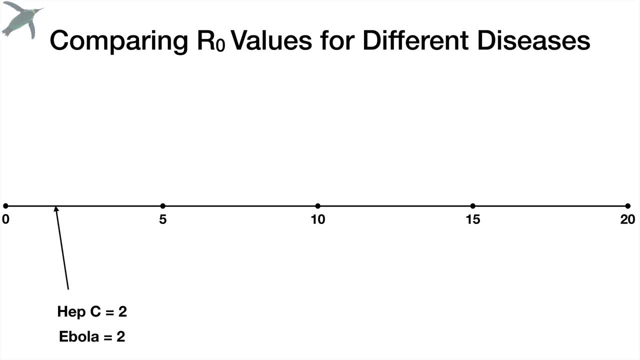 data for R-naught from the CDC website. They have great historical data. These are averages. Hepatitis C and Ebola: I'm talking about the 2014 Ebola epidemic. R-naughts reported around two SARS and HIV around four. Smallpox and rubella, seven Chickenpox and mumps. 10. Measles as high as 18.. 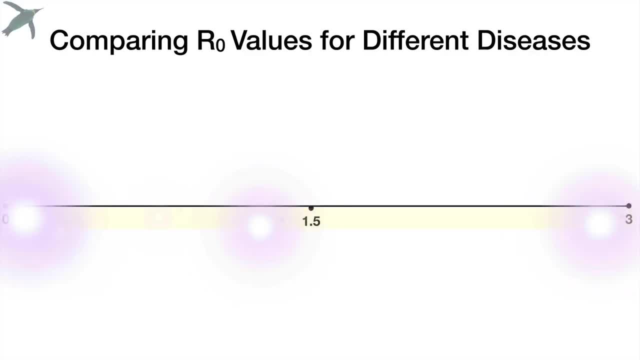 Remember this guy? Yeah, Measles. Please notice I'm expanding the lower end of this line so we can look at some more diseases down here. MERS 0.75.. And maybe now you can see how that disease kind of fizzled out over time. right, The R-naught is less than one. 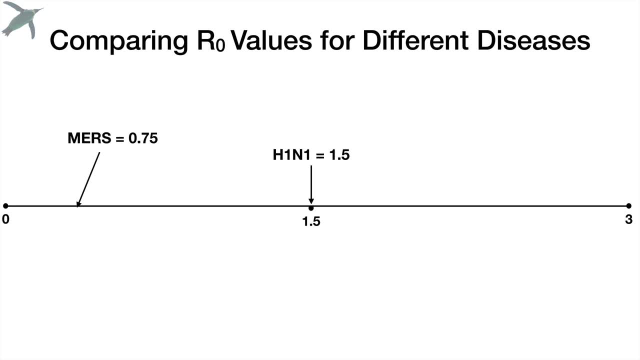 H1N1. that's the 2009 influenza pandemic that I'm talking about. R-naught of about 1.5.. The 1918 influenza pandemic: 2.2.. By the way, that was also an H1N1 virus. 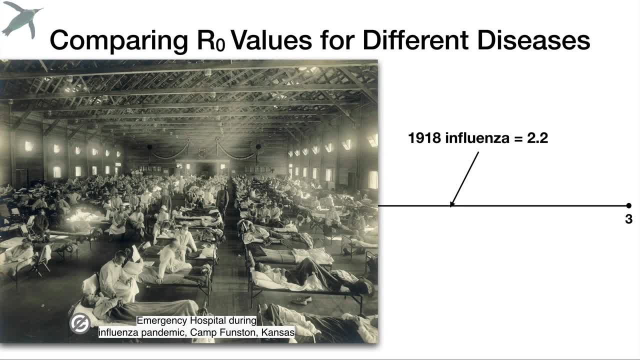 With genes of avian origin. That pandemic lasted from January of 1918 until December of 1920 and an estimated 500 million people became infected. That's about a third of the world population. The number of deaths estimated at about 50 million, Although people think that that number is. 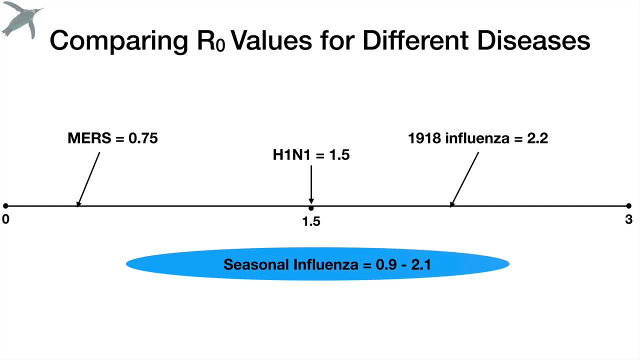 drastically under reported Seasonal influenza ranges between 0.9 and 2.1.. And COVID-19 is coming in right now at between 2.0 and 2.0.. And the R-naughts are一 And I'm talking about these patients. 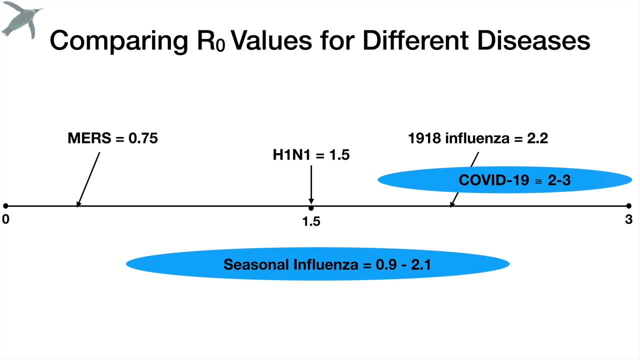 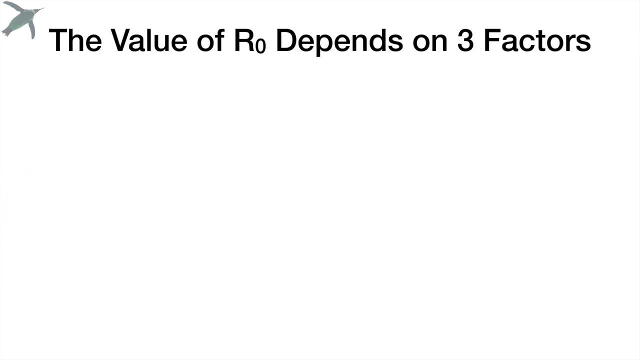 And right now at between two and three. that number is expected to drop as we get more data and more people globally are tested. Now the value of R0 depends on three factors. The first one is the duration of infectiousness: How long can an infected person give the disease to other people? 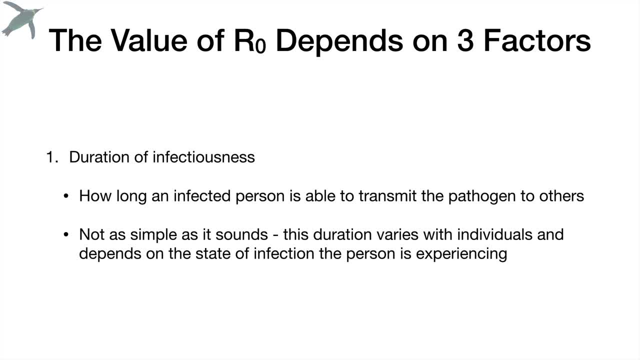 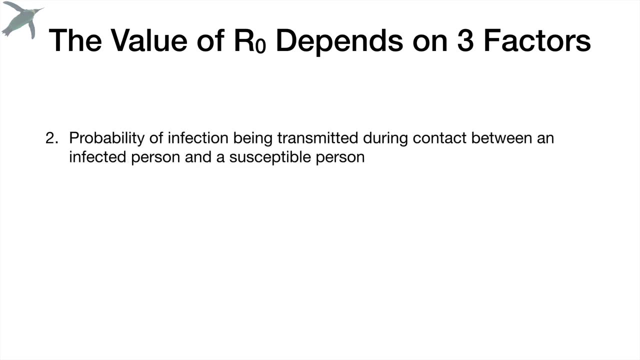 That's not as simple as it sounds, because it varies, it seems, genetically with individuals and it depends on the state of infection that the person is experiencing. We know that at different stages of infection, people shed different amounts of viral particles. Factor number two: the probability of transmission. 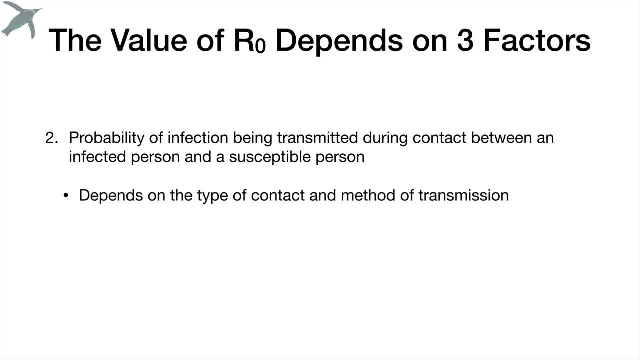 between an infected and a susceptible person. Now that depends on the type of contact and the method of transmission of the pathogen. So R0 is going to be higher when you're looking at diseases with droplet or aerosol transmission and it's going to be lower when transmission requires an. 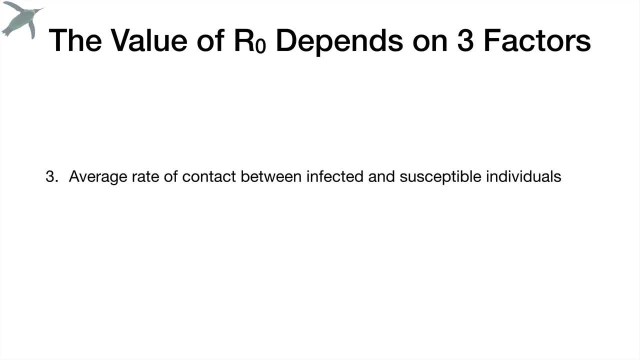 exchange of pathogen. So R0 is going to be higher when you're looking at diseases with droplet or aerosol transmission and it's going to be lower when transmission requires an exchange of bodily fluids. The third factor has to do with the average rate of contact. 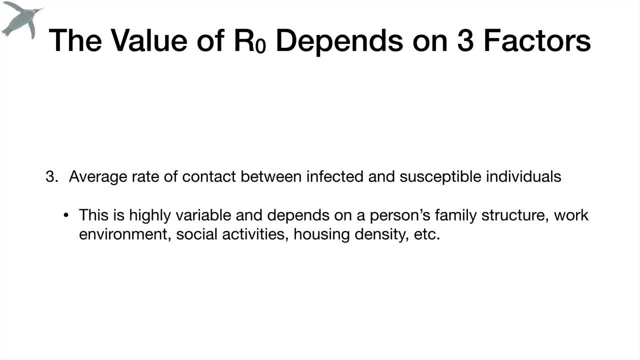 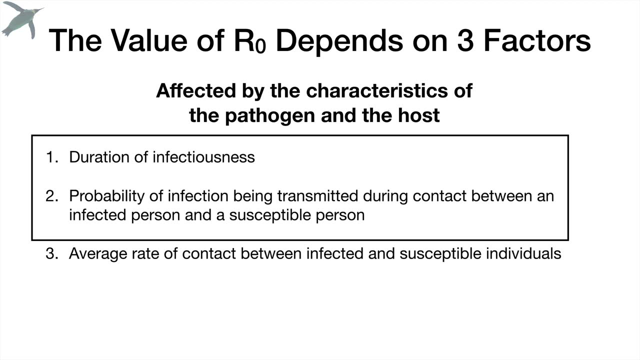 between infected and susceptible individuals. This is really variable and it depends on what kind of lifestyle, what kind of living situation, work environment and social activities, et cetera, that an individual has. So here we go. The first two factors are affected by the characteristics of the pathogen and the host. 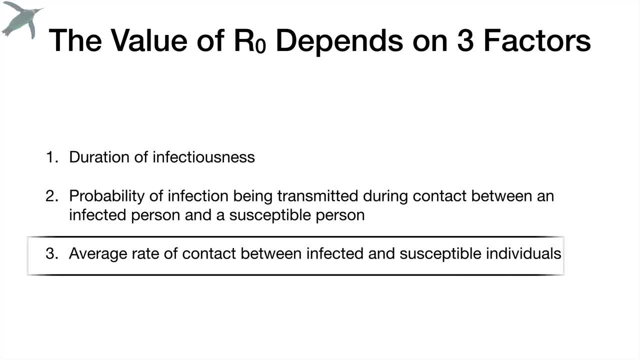 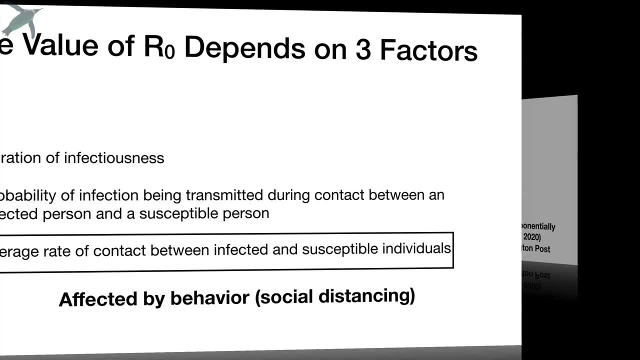 meaning that's determined by biology. This third one is the rate of infection. This third one: this is affected by behavior, and that's where things like social distancing play their role. I'm going to recommend you guys check out this incredible simulation online. 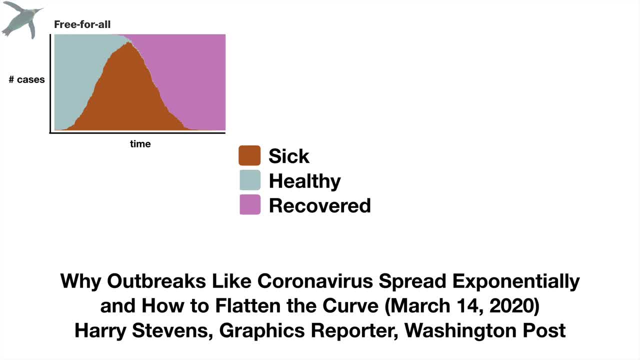 the link is below, by Harry Stevens, who's a graphics reporter at the Washington Post. He gave me permission to show the simulation in this video, but the Washington Post demanded $1,000, so I couldn't afford that. So unfortunately, you're going to have to look at this little image here. 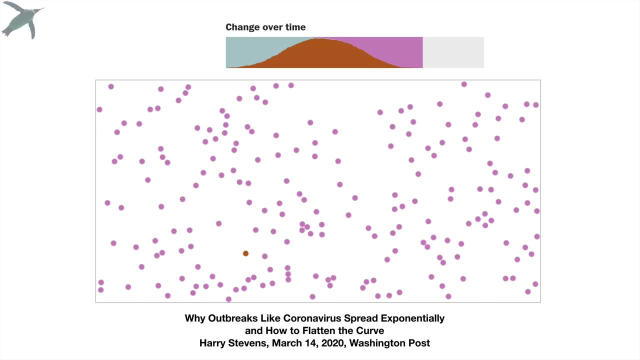 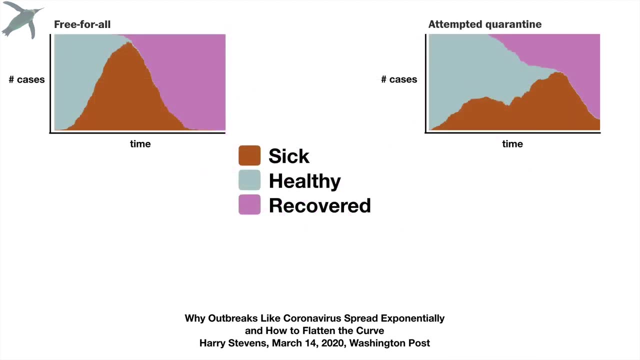 What you do when you go to this site is you can run these simulations and you can see the effect of different types of distancing on the number of cases and how they change over time. So we've got sick, healthy and recovered individuals in a free-for-all attempted quarantine. 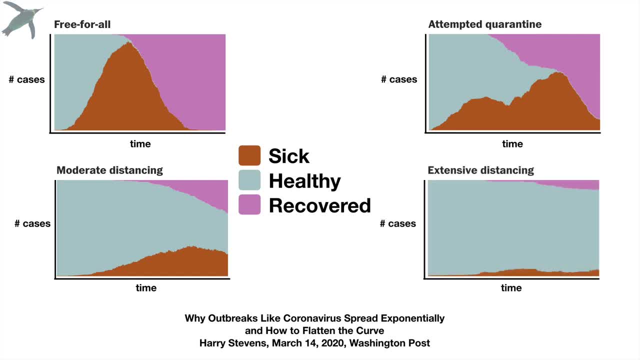 moderate, distancing and extensive distancing. Now, every time you run the simulation, your results will be slightly different. It is a really incredible simulation. Please go check it out. Obviously, this is what we're going for, right? Very, very low numbers of sick people. 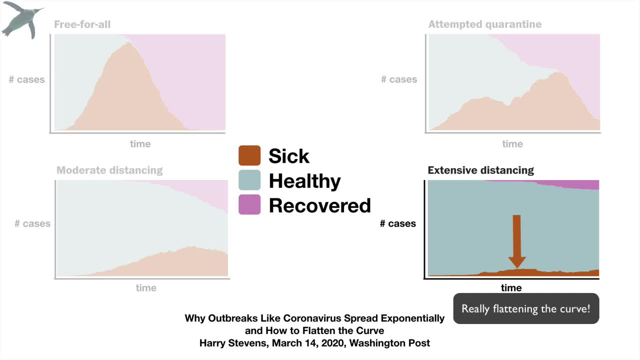 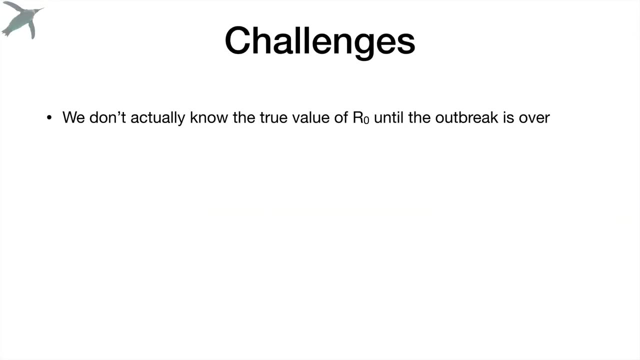 Very, very high numbers of healthy people, and this gives the healthcare system time to treat those who do become sick and it gives time to come up with therapeutic agents and, hopefully, a vaccine. Finally, some challenges here. We don't actually know the value of R-naught until the outbreak is over, and that does frustrate us. 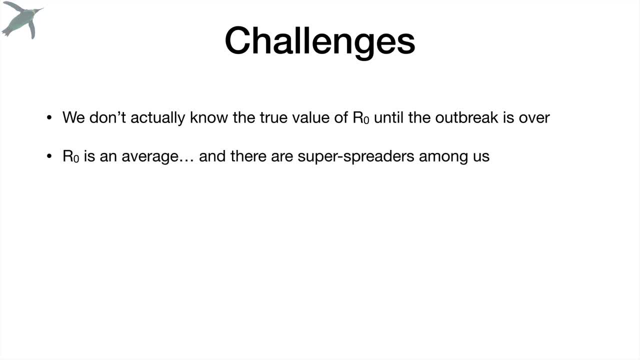 but that's just the reality of how this works. R-naught is also an average, and there are people that we call super spreaders. It's something called the 20-80 rule, So 20% of infected people can be responsible for up to 80% of transmissions. 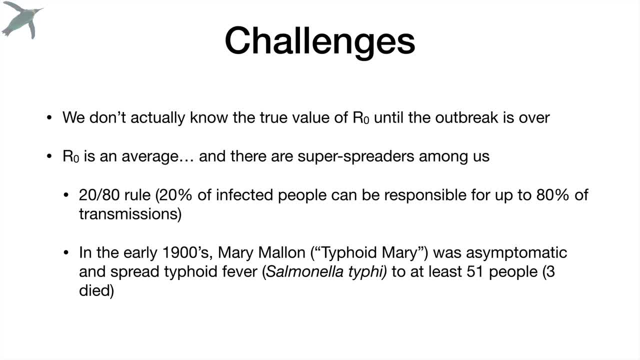 One of the most famous examples of this was Typhoid Mary. She was an Irish cook and she infected at least 51 people, three of whom died, but she herself was asymptomatic, and she's now known as a super spreader.